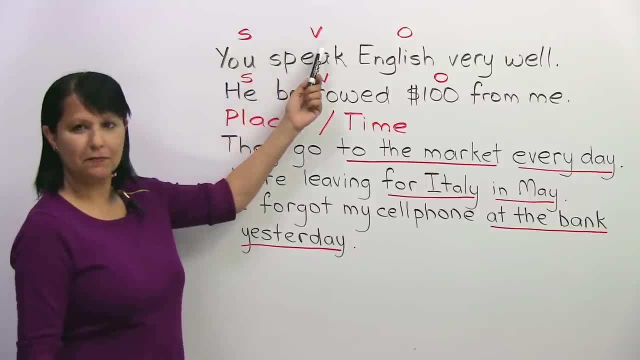 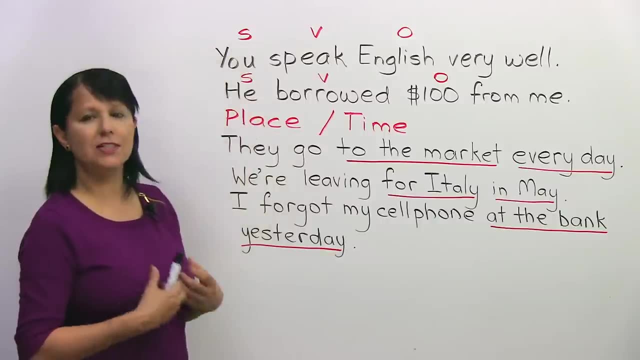 Place order: Subject, verb and object. Okay, What does all that mean? I'm going to just review it quickly for you. So the subject is the doer of the action, Who is doing the action, The verb tells us what that action is, and the object is what receives the action. 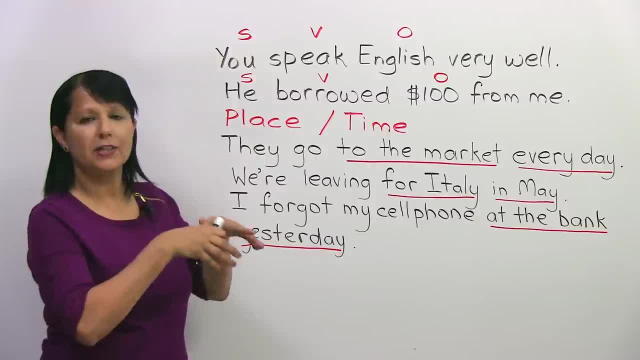 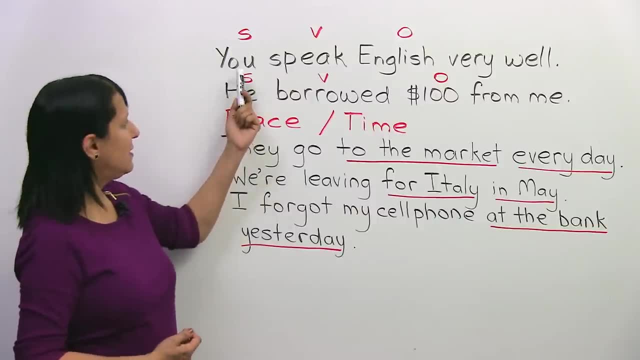 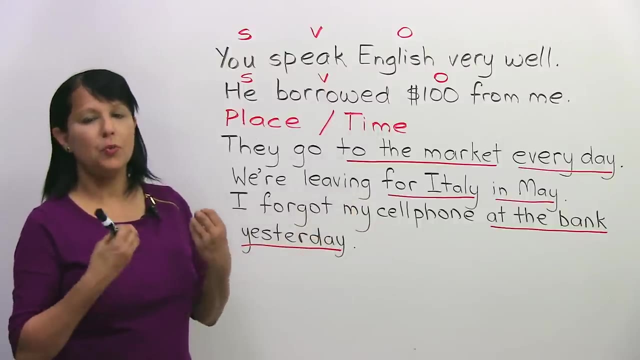 Okay. Or what the verb is doing, the action to or for, or something like that, Okay. So let's look at the example sentence. You speak English very well. That's the correct word order, because in English we expect to hear first a mention of the subject, then of the verb. 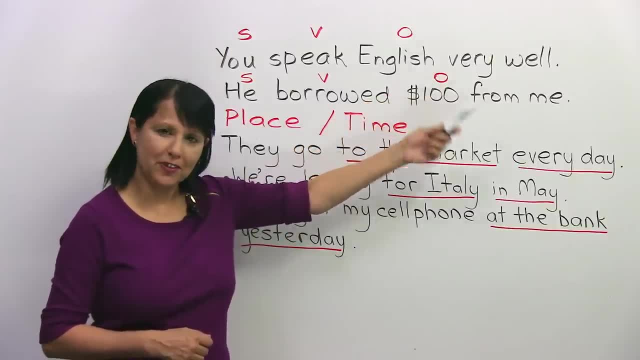 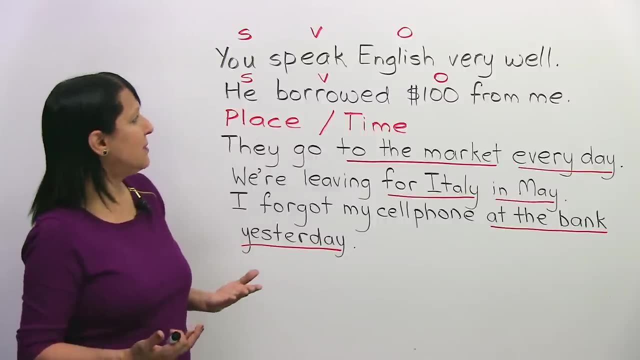 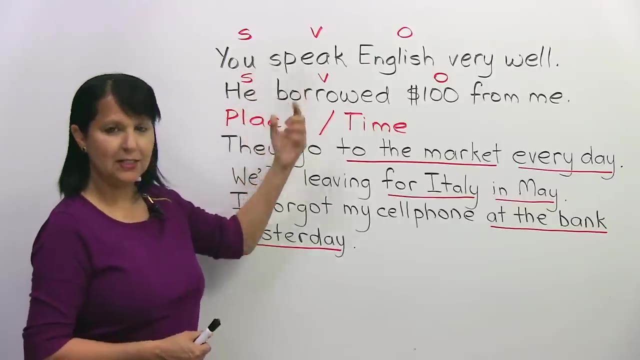 and then of the object and then after that any other information. So the mistake that students sometimes make is to say something like: you speak very well English. That's not correct, Because you speak- speak what English? And then any other details, like: very well. 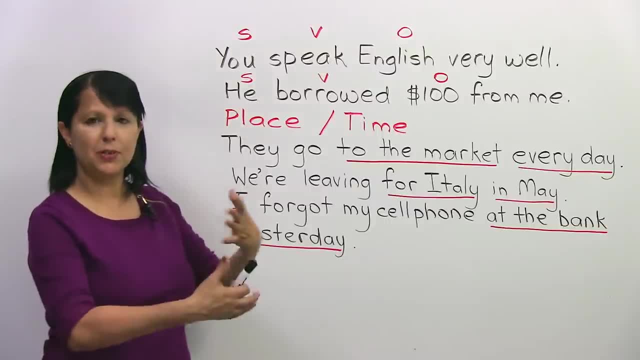 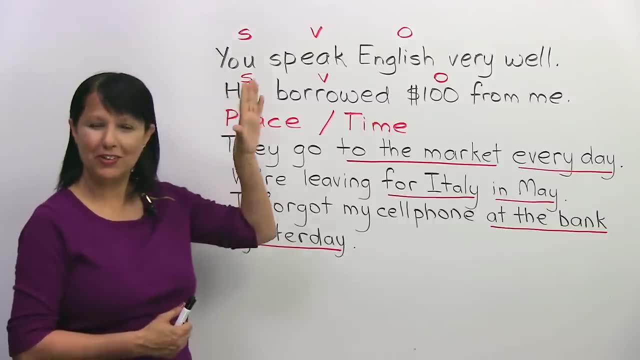 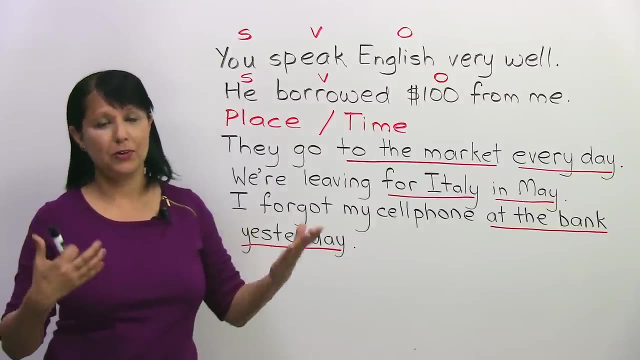 So this is the basic rule. Okay, There's a lot of details that we can go into about subject-verb order. You need to know it, And if you don't know this basic subject-verb order really, really well in your sleep, then please watch our English lesson on basic word. 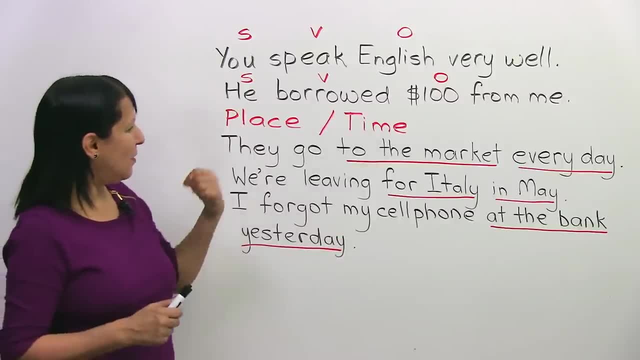 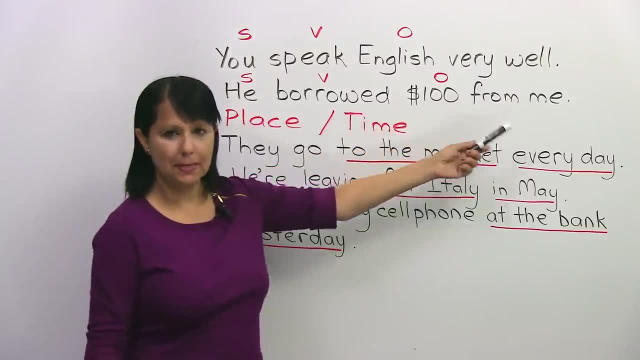 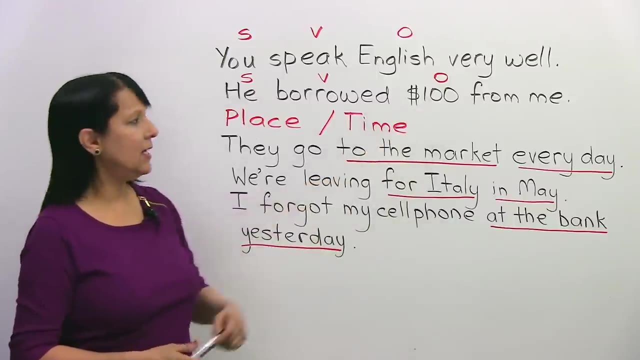 order in English. Okay, All right, Now let's look at another example Of that basic order. he borrowed a hundred dollars from me. He is the subject Borrowed, is the verb Borrowed what? A hundred dollars? And then any other information From me. 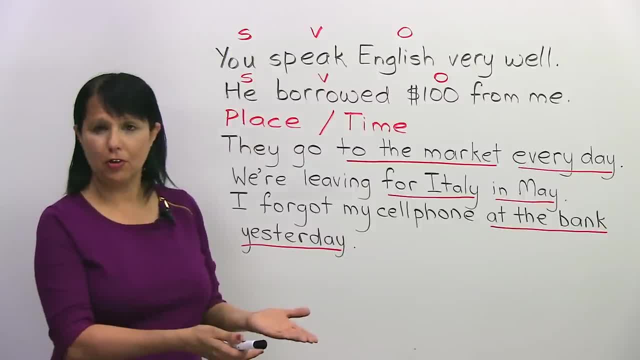 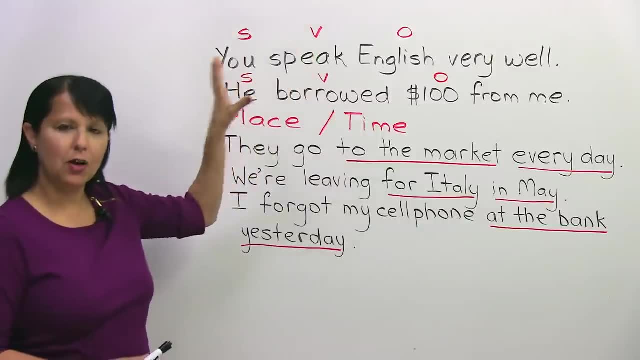 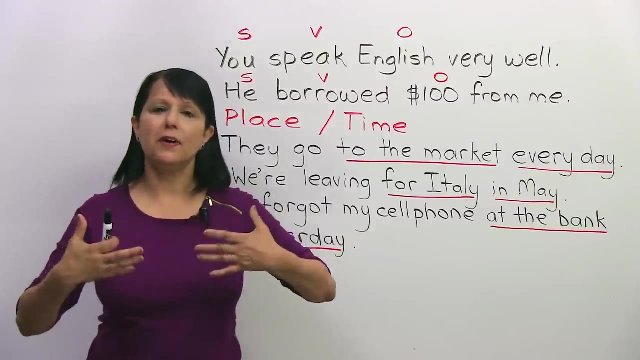 So we do not say he borrowed from me a hundred dollars. We need to say he borrowed a hundred dollars from me. Okay, Again, that's the review of a basic subject-verb order that English sentences follow. But what happens when we have other information in that we? 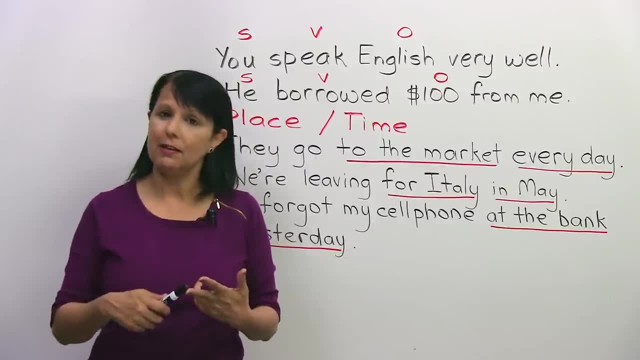 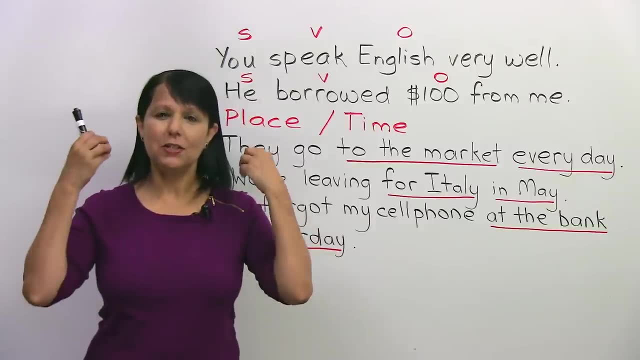 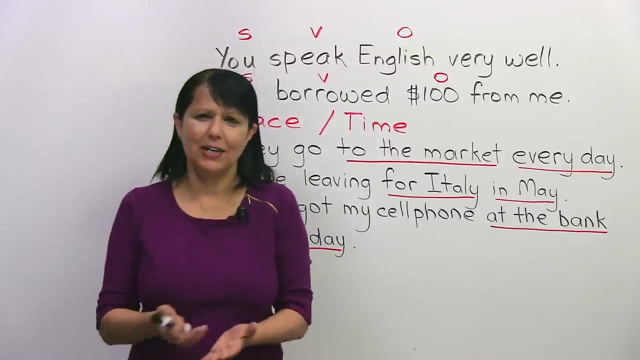 need to communicate. that's related to place and time. What do we say first? Is there a pattern? Does it matter? Yes, it matters, Because English speakers expect to hear things in a certain order. Now, if you stop an English speaker on the street and ask him in a sentence, 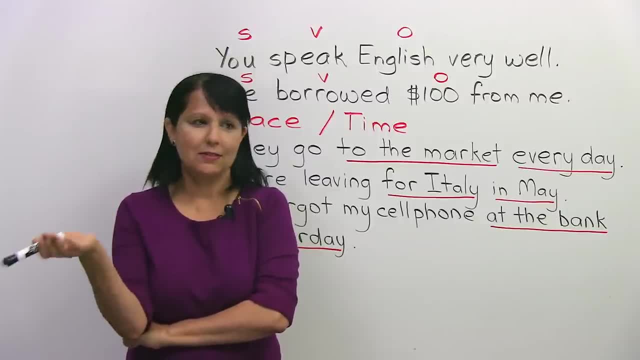 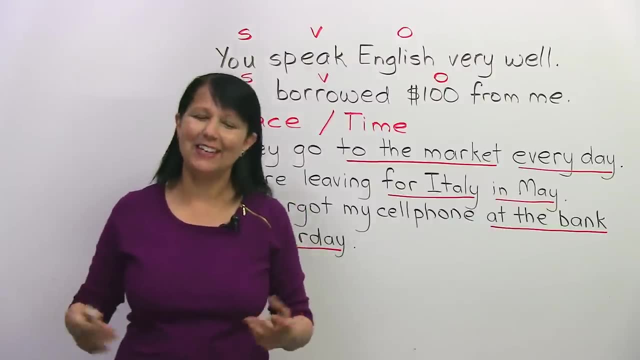 do I say place first or do I say time first? They're going to look at you like I don't know. I just say what I say, So they don't know that. Okay, When you speak a language, of course, you're not always familiar with. 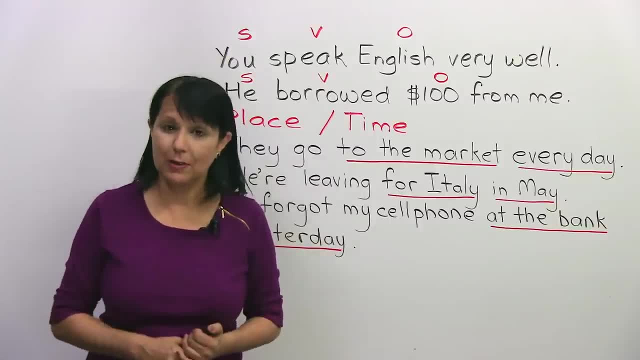 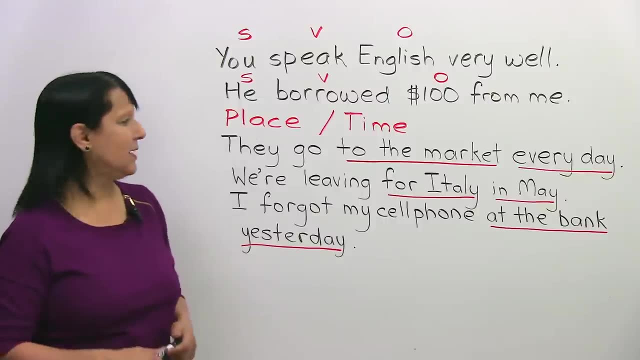 all the grammatical rules that you're following and the same in your language, Right? But as a grammar teacher and as an English teacher, I'm telling you there is an actual order that we follow normally. So this is what it is, And by learning it you can sound more. 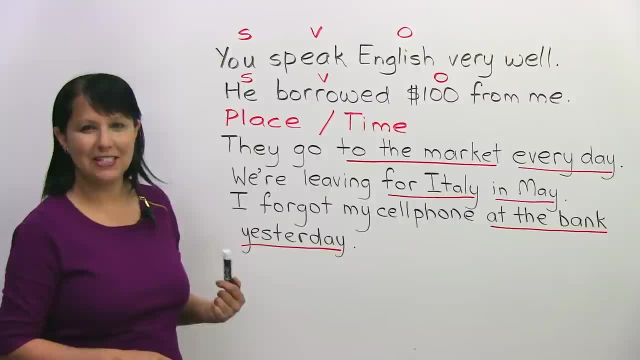 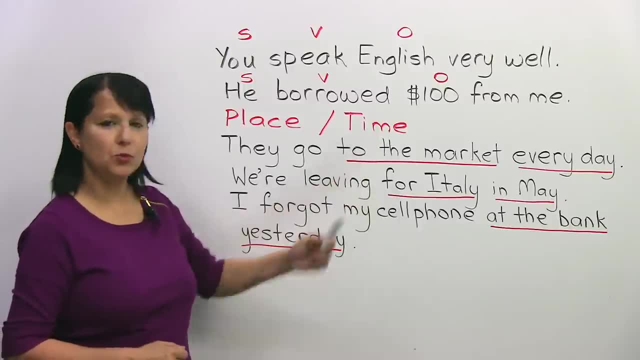 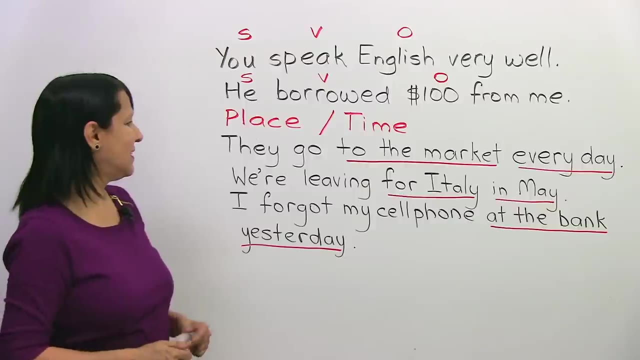 natural yourself. Okay, So the rule is this: That if you need to mention information about place, first mention that and then afterwards mention time. So place first, then time Got it. Let's look at some examples. They go to the: 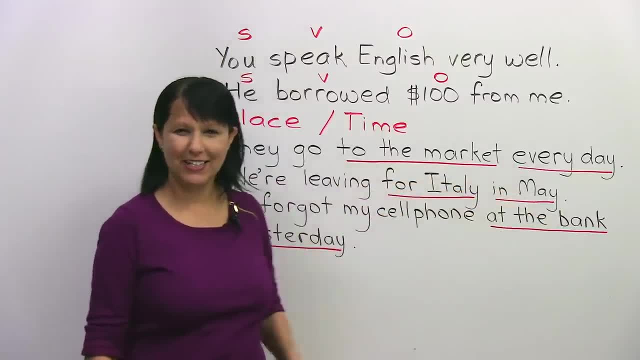 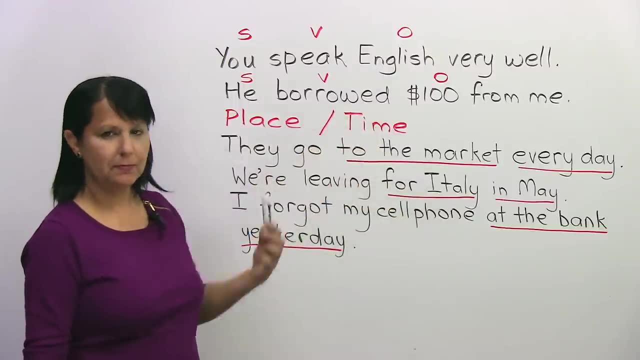 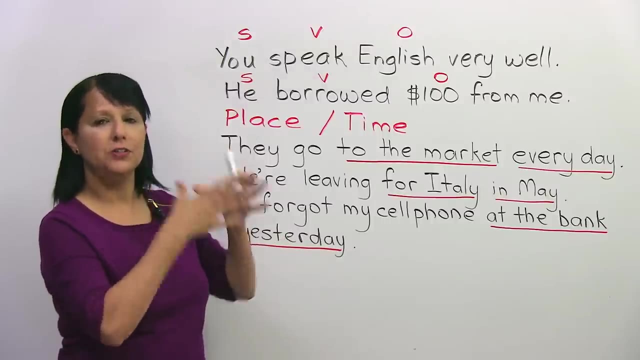 market every day, Okay. So what happened here? Where's the place? The market. They go to the market And where's the time? Every day, Not, they go every day To the market. They go Where? To the market, When? Every day. Okay, Where and when? 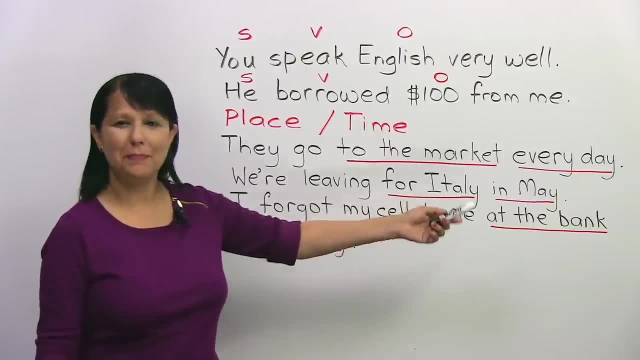 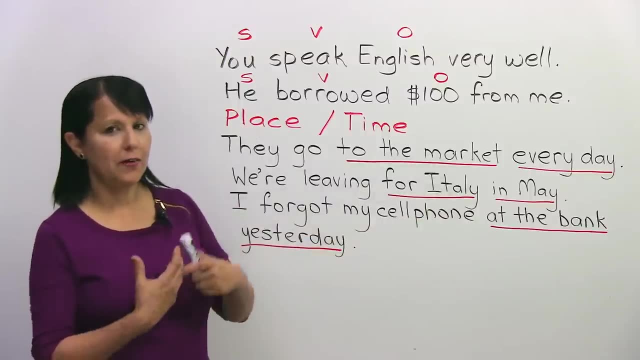 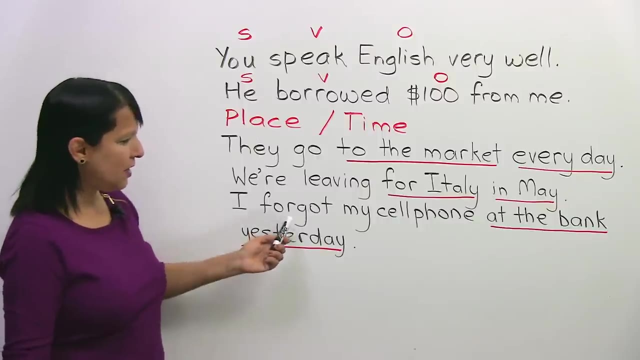 Next, we're leaving for Italy in May. Okay, Leaving for where? For Italy? When? In May? All right, Where and when. Place and time. Okay, Just say that. Place and time, Where and when. Next, I forgot my cell phone at the bank yesterday. 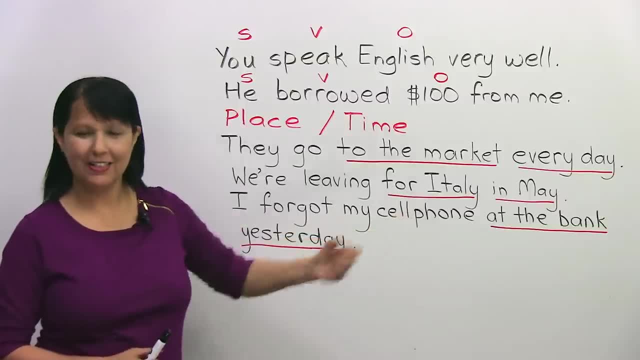 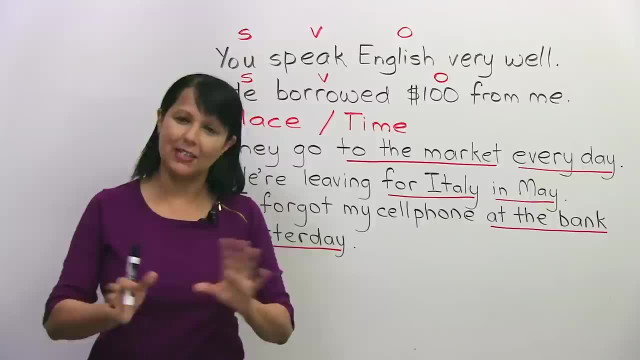 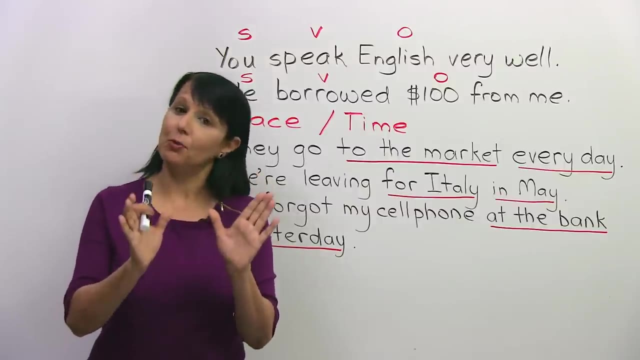 I forgot my cell phone where At the bank When Yesterday. Okay, That's really it. And even though it seems really simple, it can get a little bit confusing, So let's do a quiz to find out that you have actually understood this simple but important rule very well. 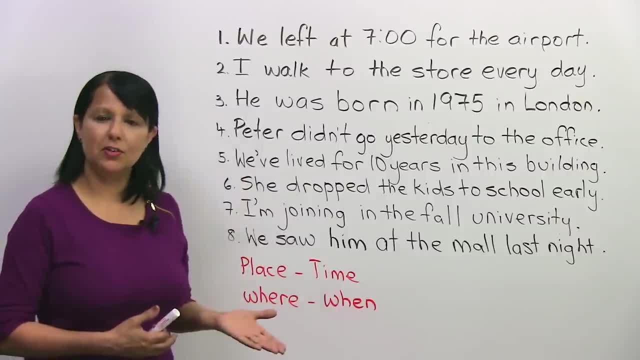 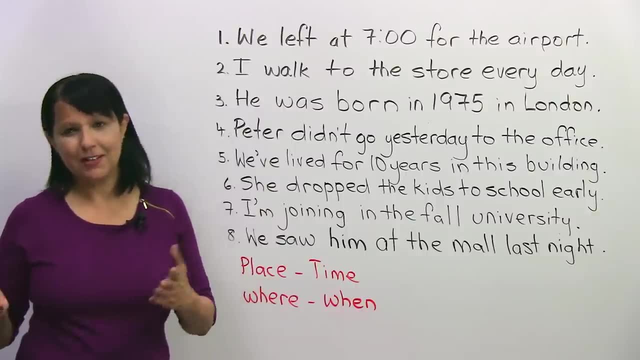 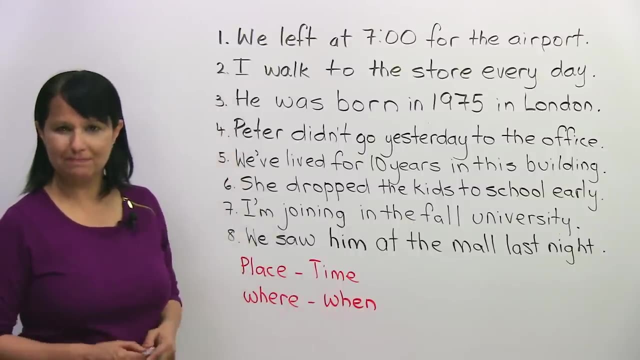 So now let's look at these eight sentences. Some of these are correct and some are incorrect based on what we have just learned about place and time. All right, So let's get started. Number one: We left at seven o'clock for the airport. We left. 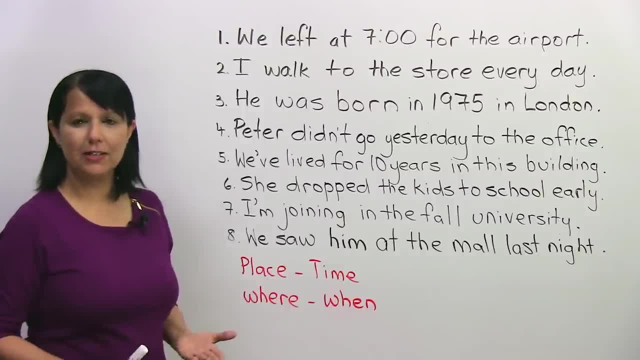 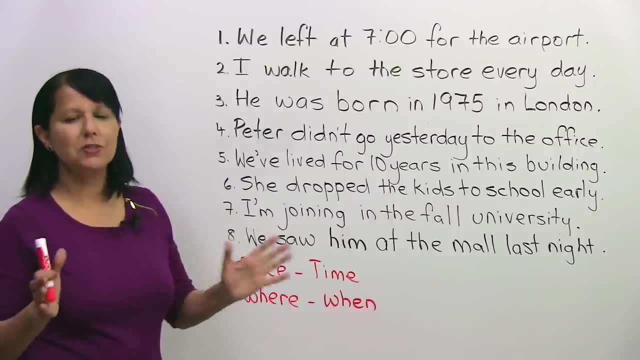 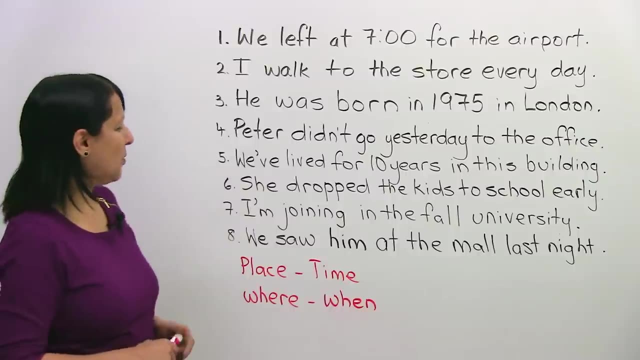 at seven for the airport. Is that right or wrong? What's the rule that we said? It's a usage rule. Okay, Sometimes English speakers might play around with it, but for you, follow this rule and it'll help you to always be right. So what's the principle Place and? 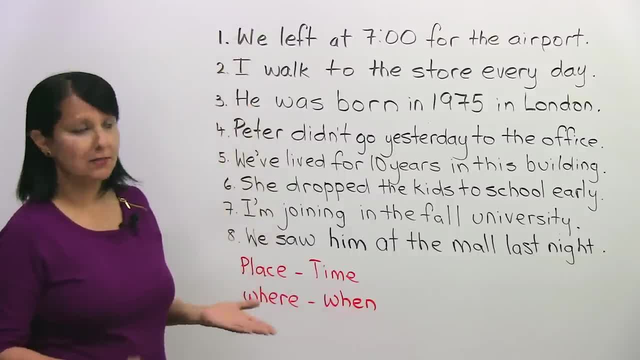 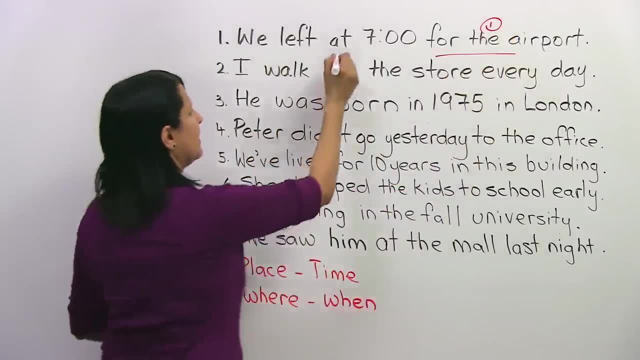 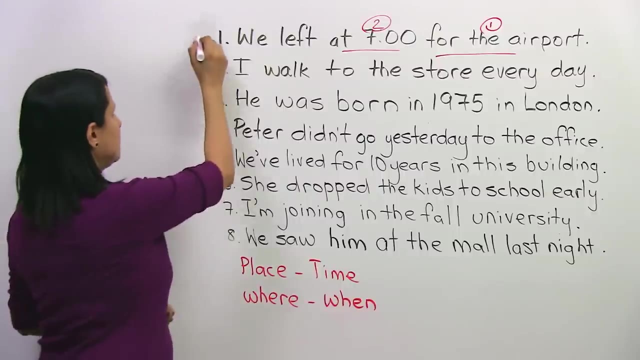 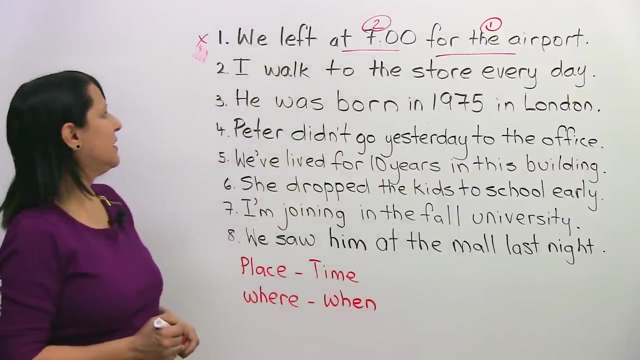 then time. So in number one, we left where For the airport When At seven. So this one was wrong the way it was, Okay. The first one was wrong. Sorry about that. Okay, So it should be. we left for the airport at seven. Number two: I walk to the store every day. 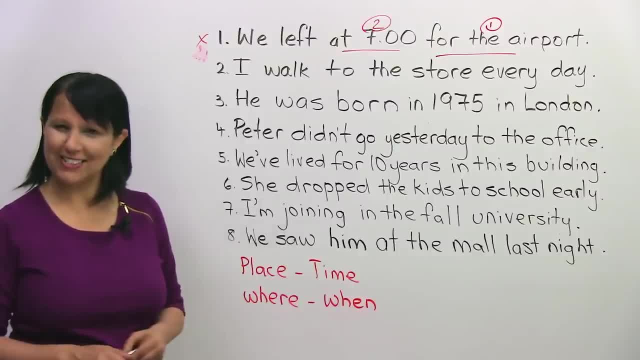 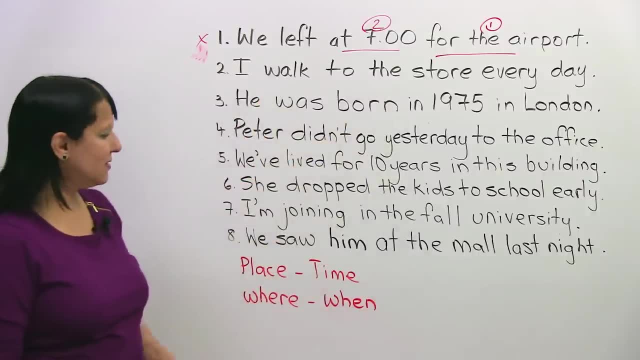 Walk to the store every day, Is that correct? Well, I walk where? To the store when? Every day, So this one is absolutely fine. Okay, Number three: He was born in 1975 in London. He was born in 1975 in London, Is that right? 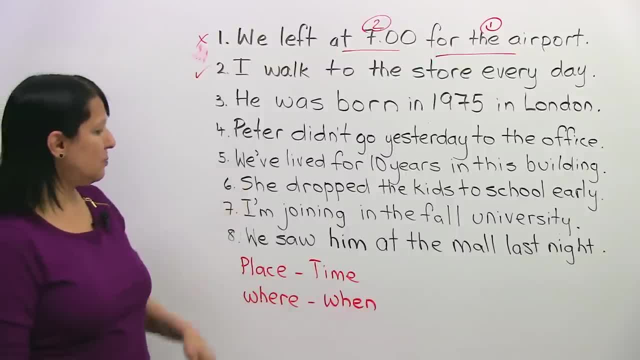 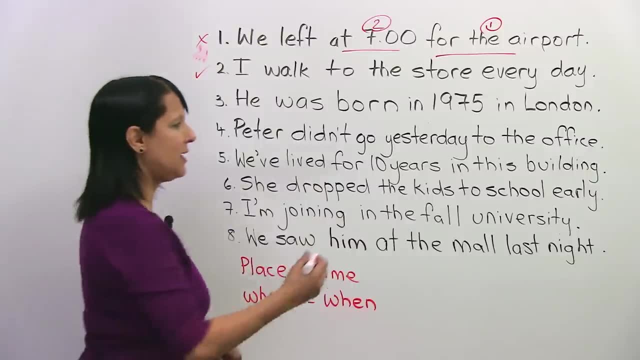 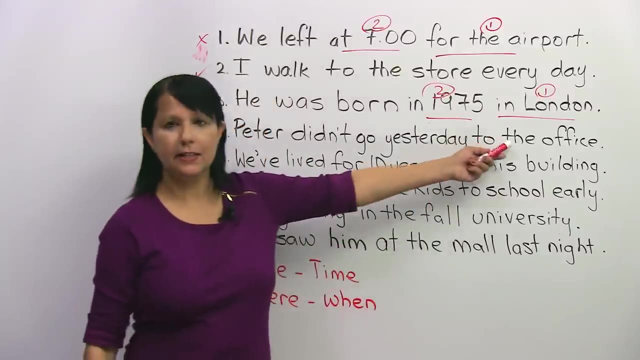 or wrong? Let's check. He was born where. Oops, we have when first, so that's not right. okay, So we should say: he was born in London in 1975, right, He was born where? In London. 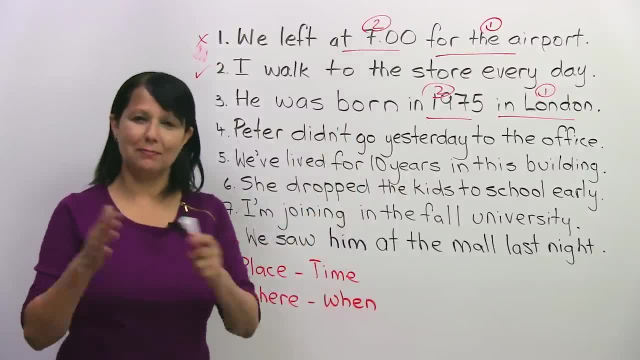 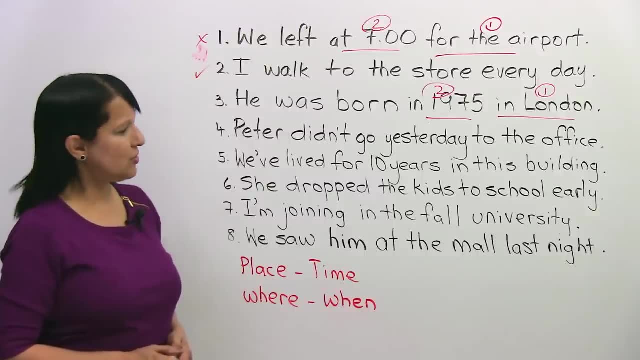 when In 1975.. Getting it Where? when? place time? okay, That's the rule we're following. Number four: Peter didn't go yesterday to the office. Peter didn't go yesterday to the office. Is it right or wrong? What do you say? It is yes, It's wrong, okay. 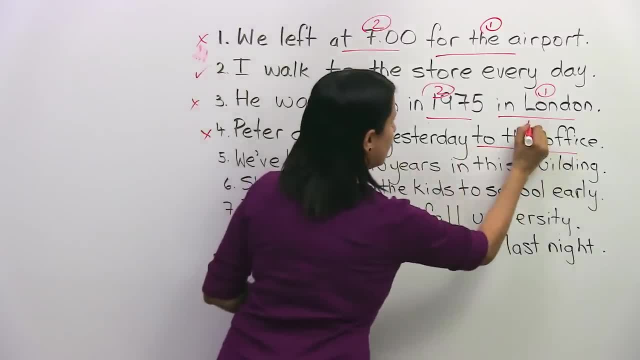 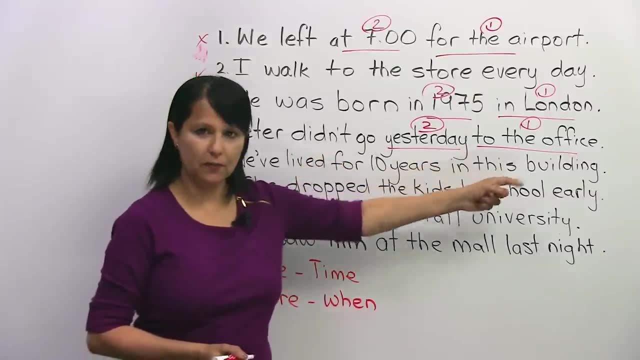 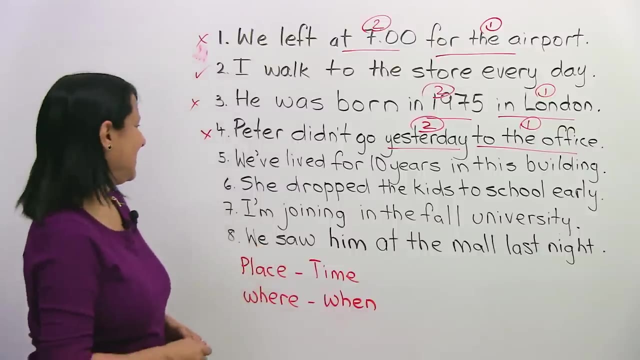 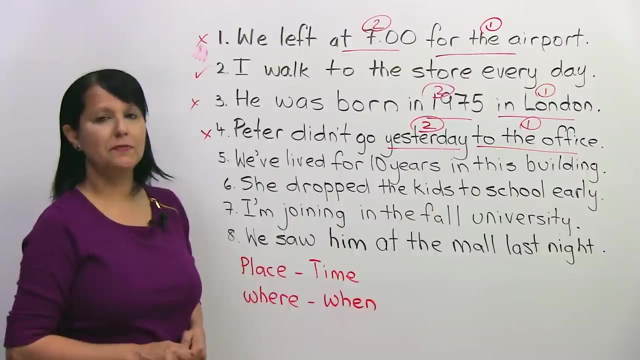 Because Peter didn't go. it should be. Peter didn't go where- To the office when Yesterday. okay, Are you getting it? Are you starting to see the rhythm of it? Number five: we've lived for 10 years in this building. We've lived for 10 years in this. 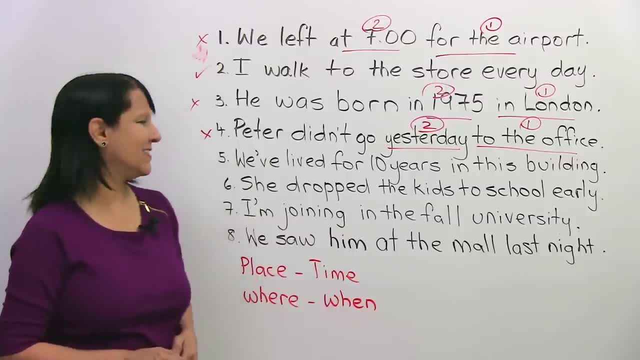 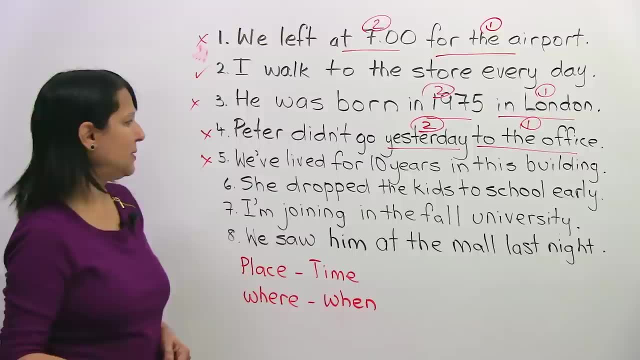 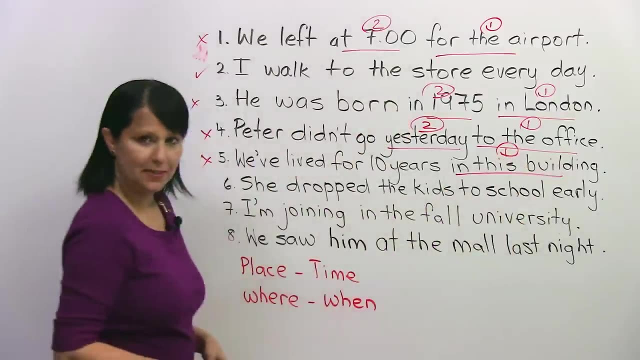 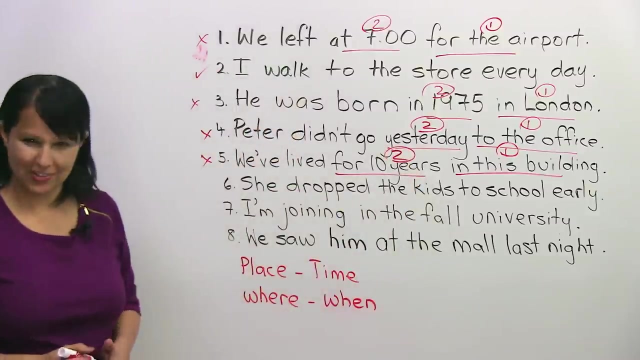 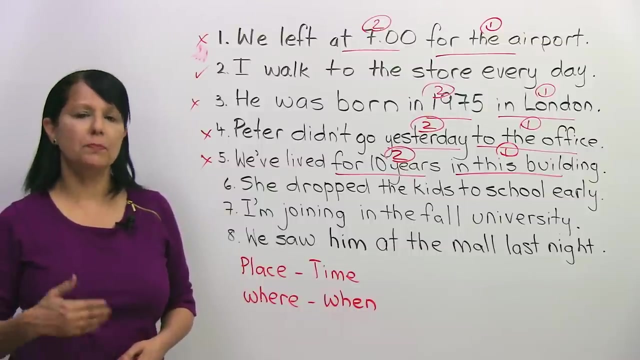 building. Is that correct or incorrect? Think about it. It is actually incorrect because we should say: we've lived where In this building time. we're talking about time when, For 10 years- okay, Number six- she dropped the kids to school early. She dropped the kids to school early. 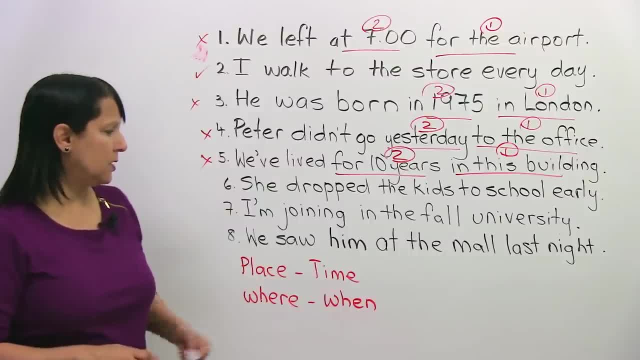 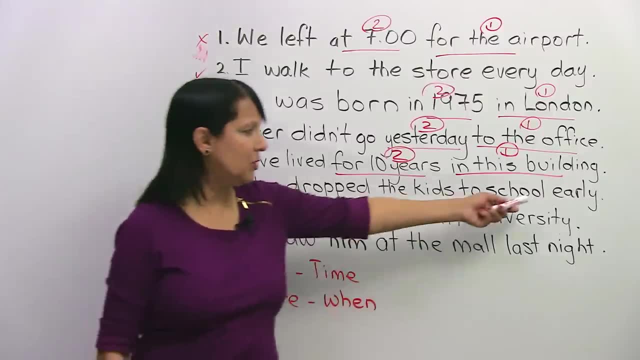 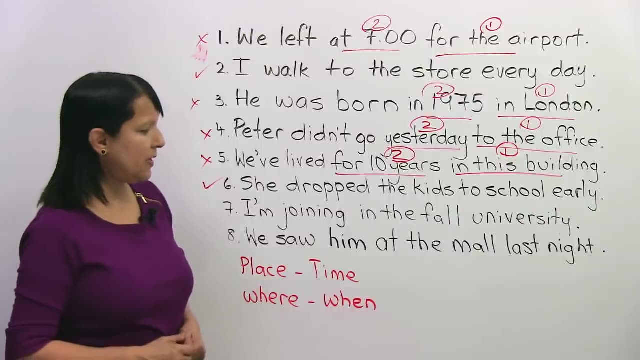 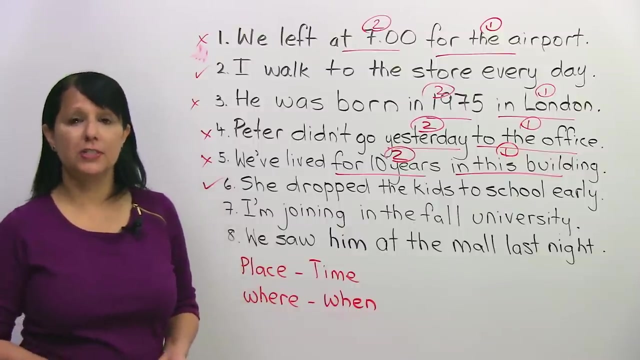 So she dropped the kids where To school when Early. So that one was correct. okay, That one's right Number seven. I'm joining in the fall university. I'm joining in the fall university, Is it? 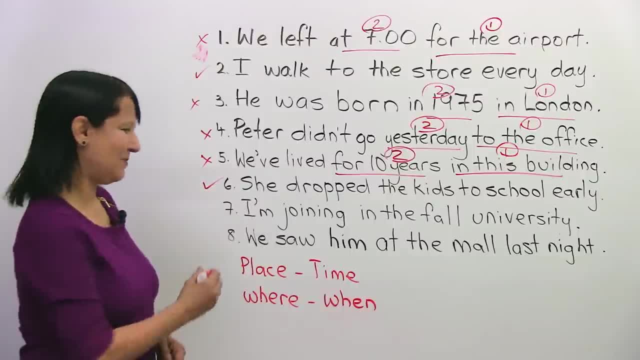 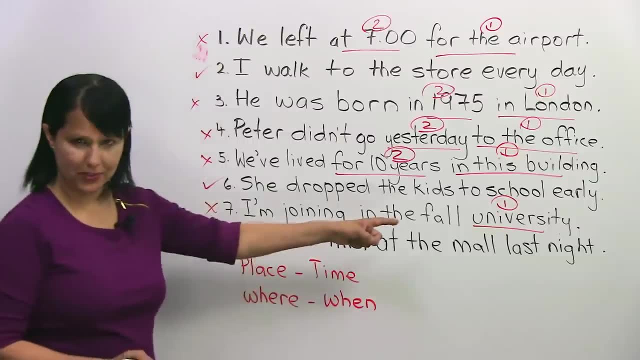 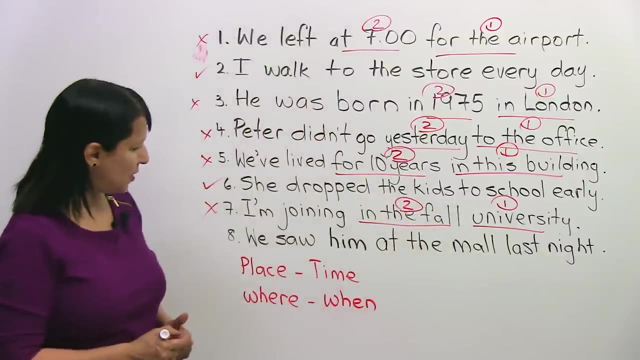 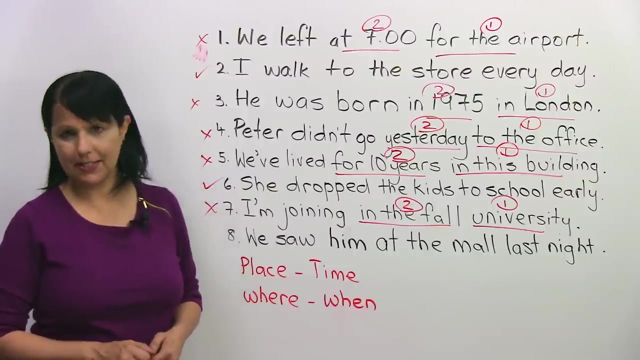 right or wrong Doesn't sound right, does it? No, No, it's wrong. So I'm joining where? Which place? University, when, In the fall? okay, Good. And the last one: we saw him at the mall last night. We saw him at the mall last night. 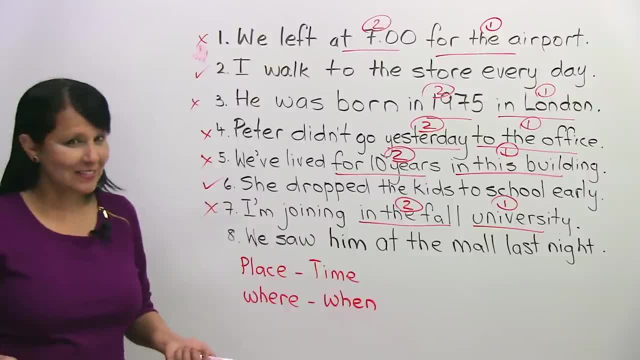 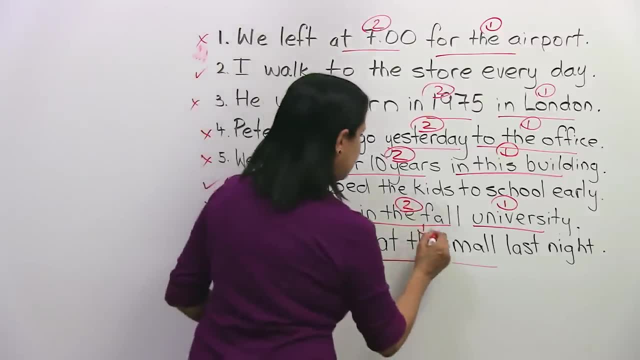 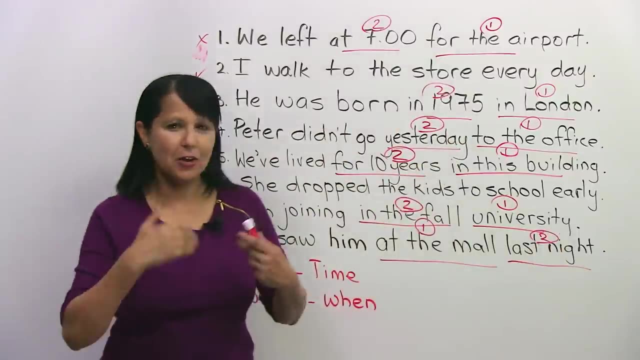 Is that right or wrong? That is actually right, Because Where We saw him, where At the mall And when Last night? Okay, All right. So I hope that by doing these exercises, by listening to the explanation of the guidelines, that 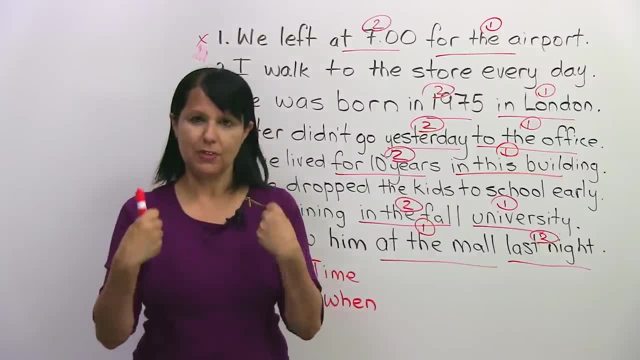 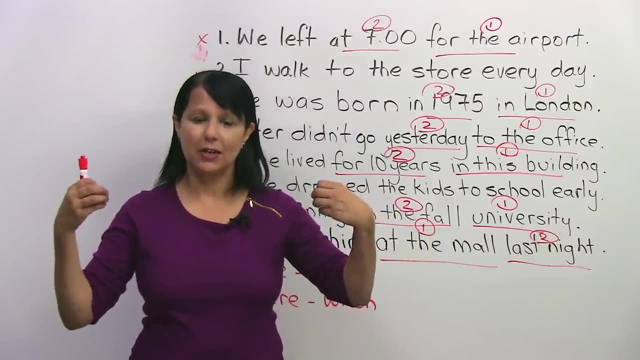 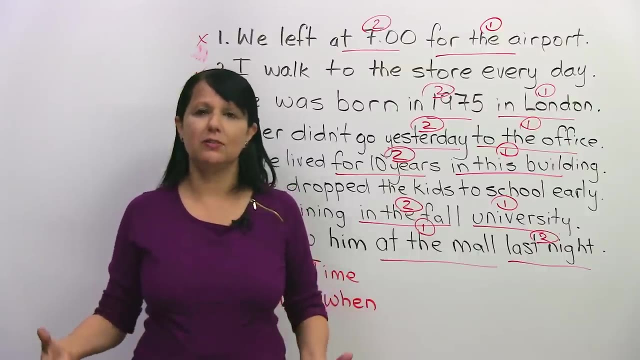 you have kind of understood and absorbed this principle of place before time. when we are constructing an English sentence, Try to remember that when you create your sentences, Try to write just now some sentences. That's the best way to do it, Not just theoretically. 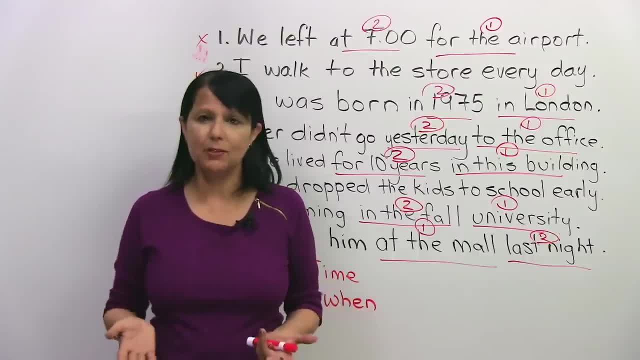 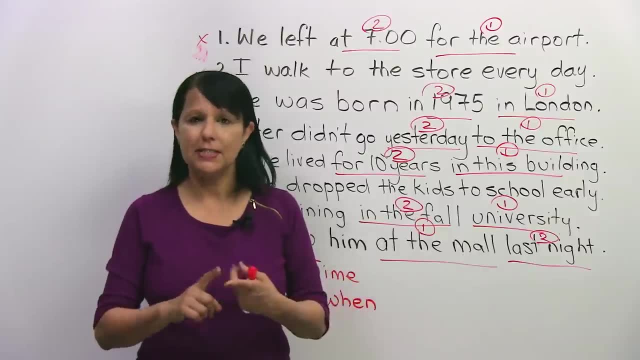 but also practically in your own life. Talk about some things happening around you, Talk about some, Write some sentences about what you did, what members of your family did, And use place and time in your own examples. That's the best way for you to remember these. 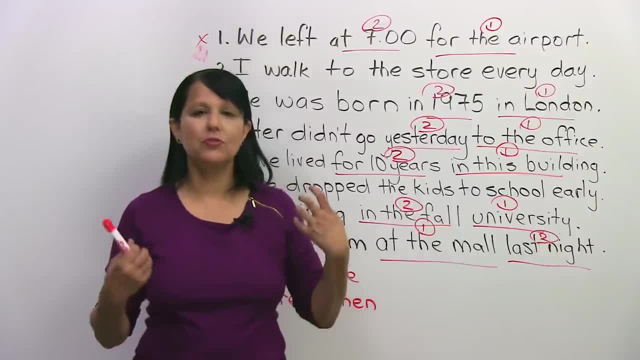 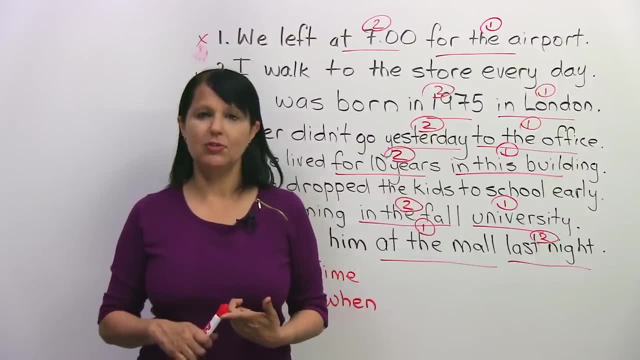 rules. okay, Now here are some other things you can do to really master this very important area. okay, So number one: go to our website, wwwengvidcom. There you can do a quiz on this and practice a little bit more. You can also watch the other lesson that I've mentioned, and there 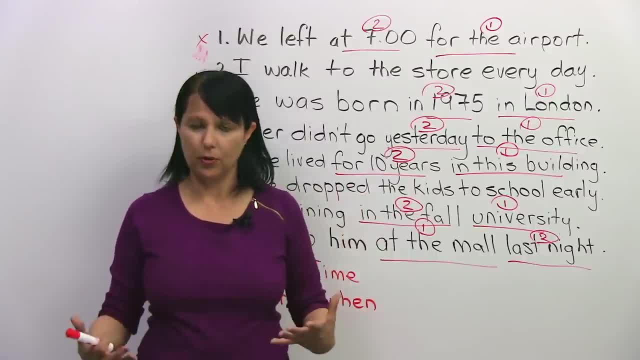 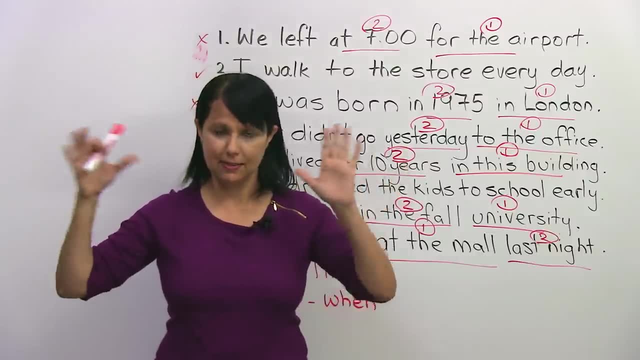 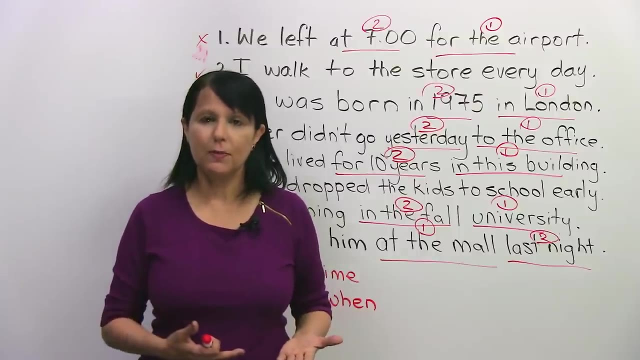 may be other lessons that have to do with word order, which will help you to really master even the basic word order- subject, verb, object- in case that's something you're not sure about. You want to really master that. Plus, you will also find on our website a free resource which you can download: a page. 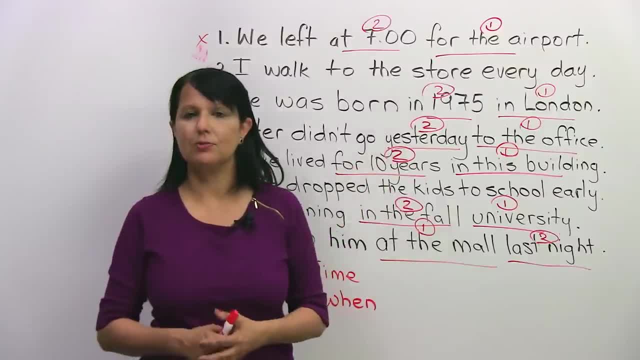 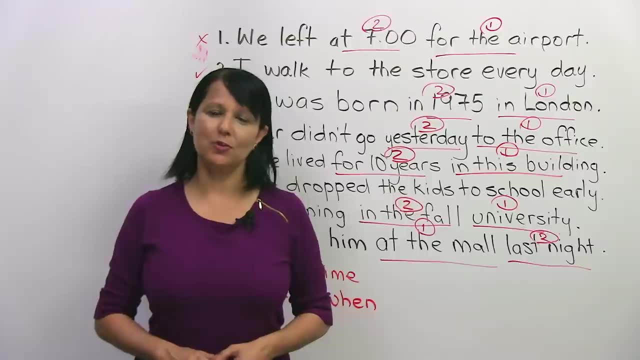 with information about this. It summarizes this subject, so please download that. I wrote that for you And, of course, please, if you haven't already, subscribe to my YouTube channel so you can continue to get lots of useful lessons, which I hope will shorten your learning. 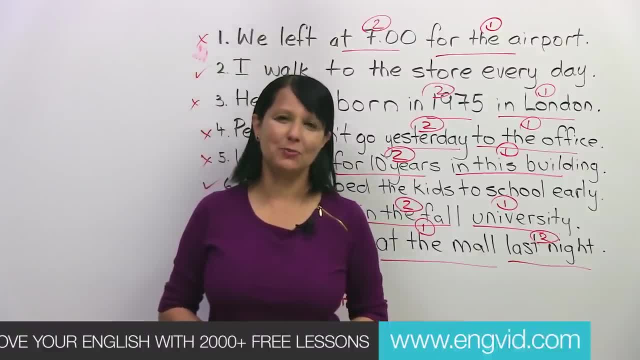 path in English. Okay, Bye for now. All the best with your English. 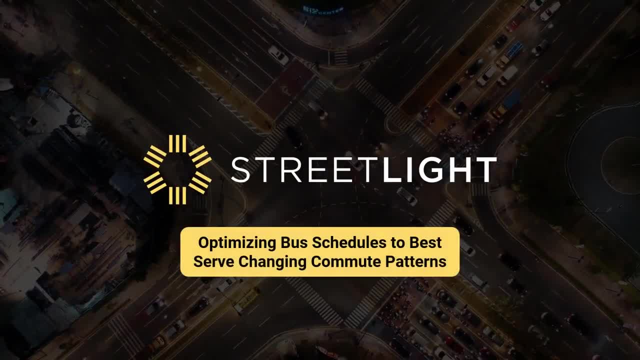 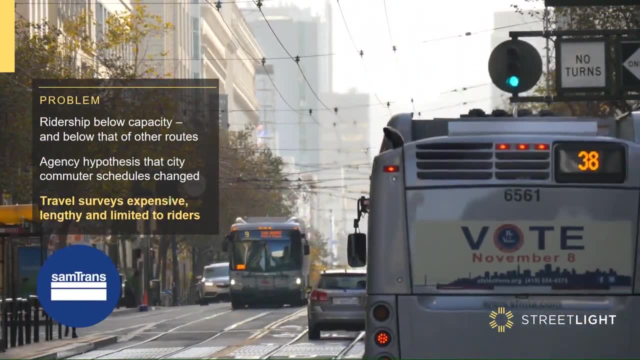 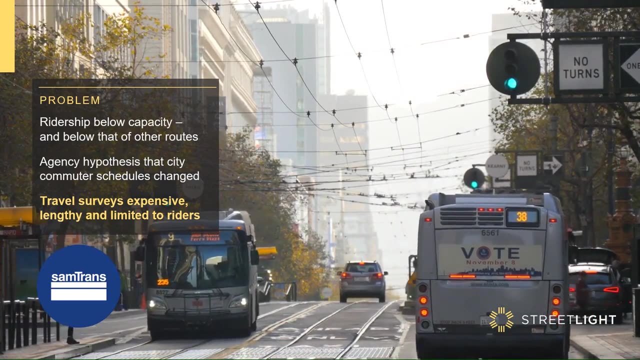 Sam Trans, a Bay Area agency, needed to respond to shifts in commuting patterns as a result of the pandemic. They sought to find out why ridership had severely dwindled on a previously popular express bus route to the city. Travel surveys are expensive, lengthy and limited to riders. 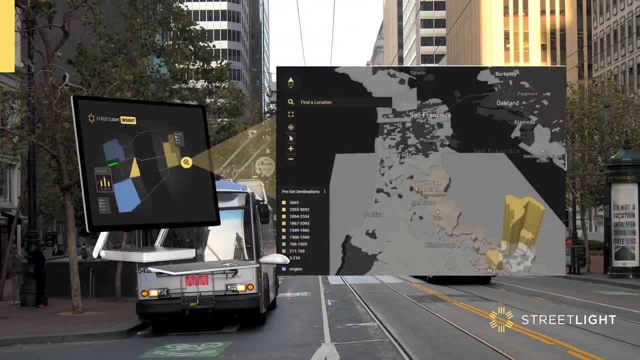 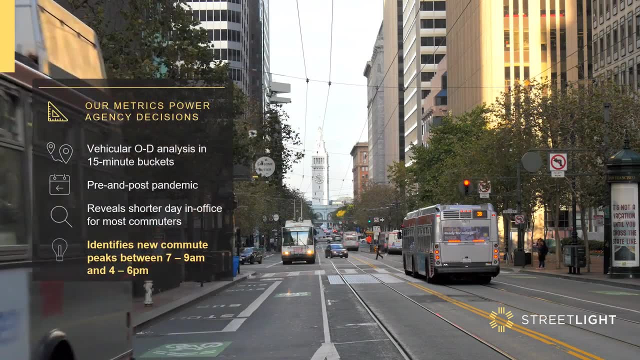 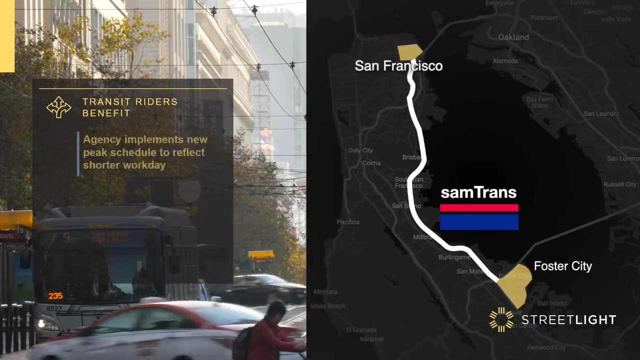 So to investigate. Sam Trans used Streetlight's origin destination vehicle metrics to understand how commute travel patterns shifted in the region. By identifying new commute peaks at 7 to 9 am and 4 to 6 pm, the agency was able to implement a new peak schedule to accommodate a shorter work.